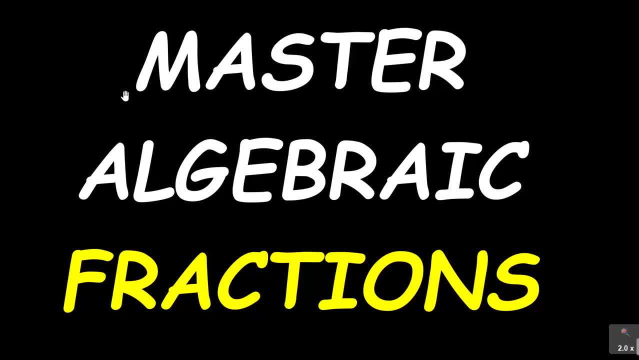 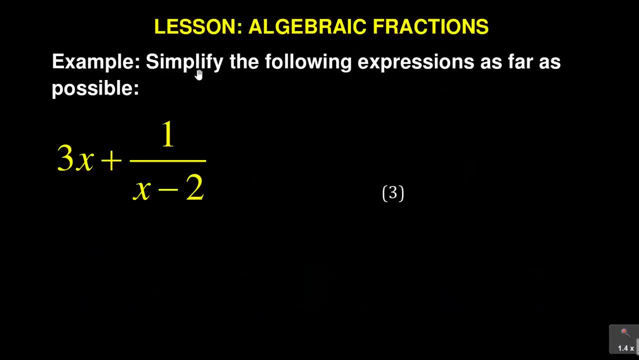 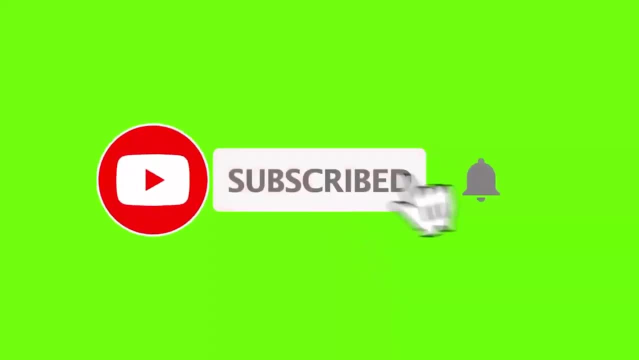 of understanding until the last one, and at that point you'll be able to follow up easily. so let's go straight to the lesson. the first lesson is: you say: simplify the following expression as far as possible, and there is a fraction given which is three x plus one over x minus two. you're supposed to simplify now whenever you're dealing with. 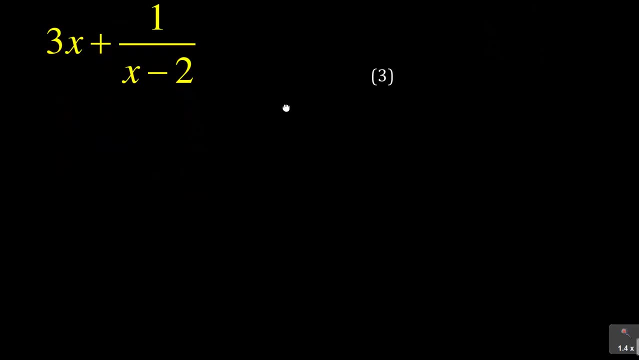 fractions just to give a little bit of foundation. as i say, if i'm to say, for example, i want to add two over three plus one over two plus three over five, i'm just giving an example. now, how do you go about this? what is most common? 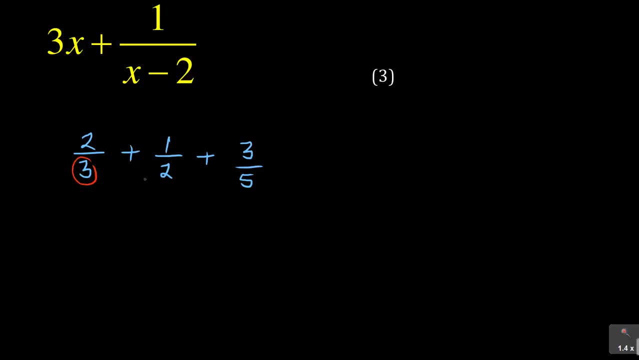 is for you to find the low lowest common uh multiple or the highest, um, actually a common denominator. let me use the great common denominator so that i don't confuse myself also. so we're going to use: look at the highest common denominator, which is the hcf of three, two and five. 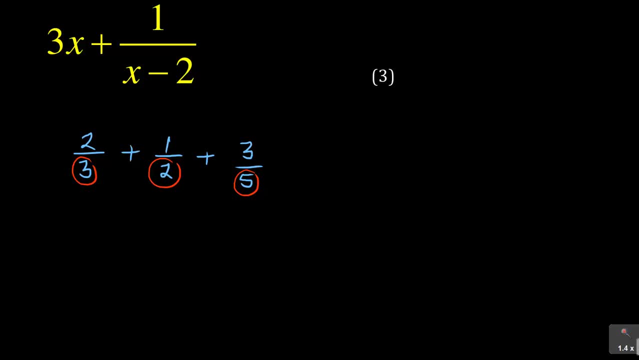 so that is what is your focus. but i have a way sometimes that avoid the whole thing, of looking either at the lowest common multiple or at the highest common factor. so what i do is i look at this denominator, as i just said, i look at my three, i look at my two and i look at my five. so i'm 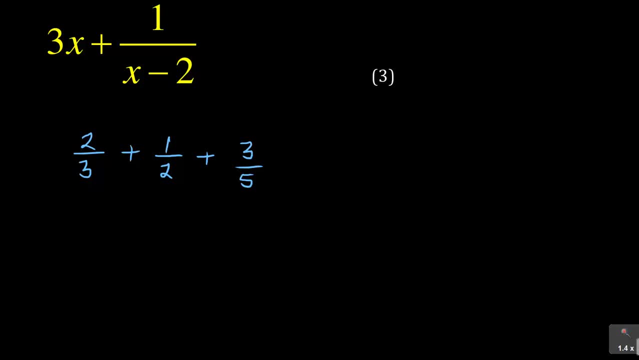 going to take them as they are and write them down as three and put a bracket. i have my two, i put a bracket, i have my five. so this is what i do. and then the next thing is: why am i choosing? where am i getting three to five? i'm getting them from these denominators. as i said, it's obvious. 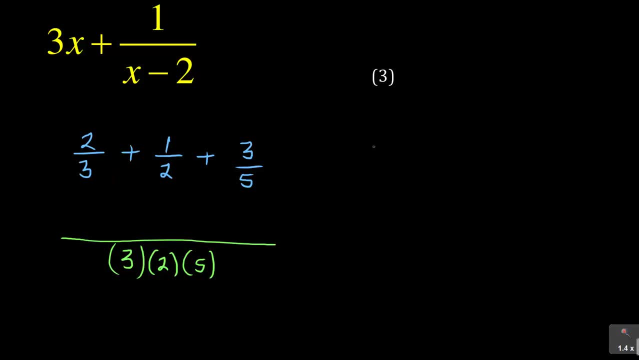 right now. how do i then solve this particular fraction? so what i'm doing is i'll start with the first one here. so what i'm saying is i'm saying three into three, two, five. so i'm going to have my three, my two and my five and i'm going to divide it by that particular denominator. so i'm 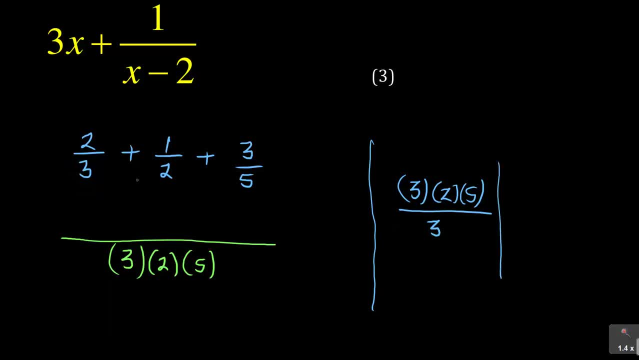 going to say over three. i do the same thing with the other one, which is three, two, five. now i'm going to be dividing by two in this case, so it's over two. i do the same thing: my three, my two and my five, and i'm going. 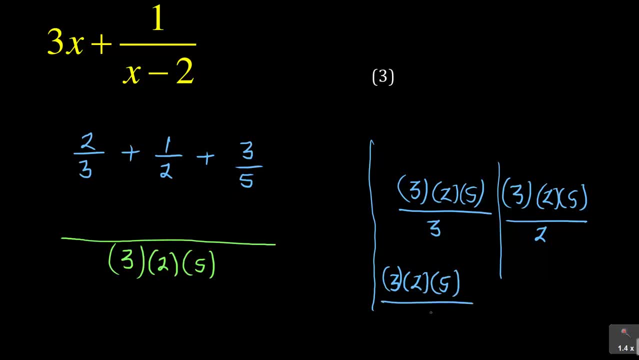 to be dividing this time by five. so this is basically what i'm doing in each and every fraction. so when i cancel out, you can see the numbers that are remaining in. the first one is two five. so that's what i'm going to write. i'm going to write two five. now, when i've done that, i must multiply by the top, which is the. 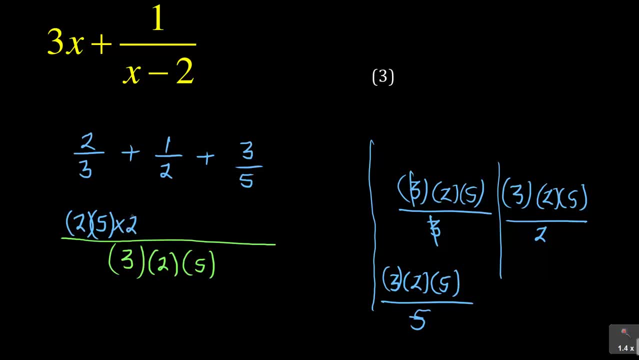 numerator and then, which is times two, you can also actually put it in fraction and say bracket two. and then i go to the next one, which is a plus. i do the same now. it's one over two. um, that i'm focusing on, remember this particular two. here is what i have on this particular side. so i'm 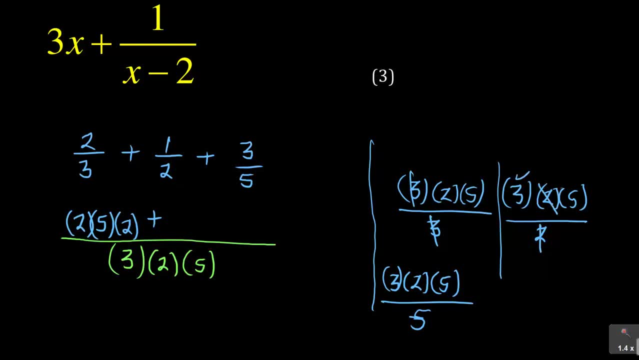 canceling the two. that cancels the two and what is left is three and five. so i'm going to write the three and the five. it is going to multiply by the top there, which is times one. follow again plus. i do the same thing. the five now is the one that i'm focusing on. so five will cancel the five. i'm. 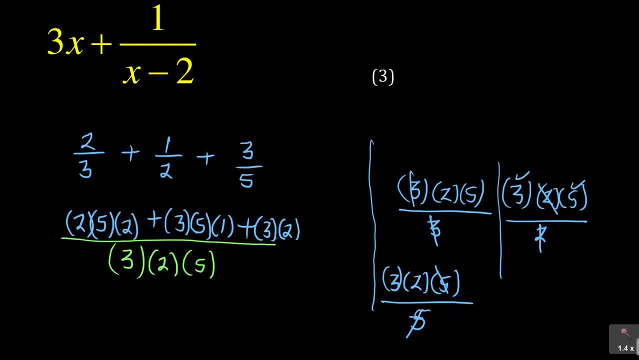 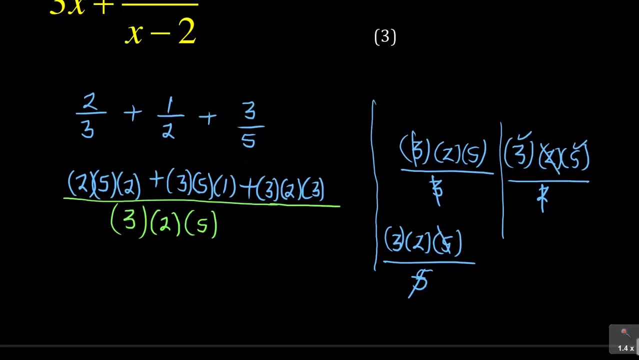 left with three, with two and um. after that i'm i'm going to multiply by the top, remember, which is three. so basically, this is what i'm having and if i continue to simplify this, this will be equal to. then you start multiplying with the calculator: which is two times five, which is ten, ten times. 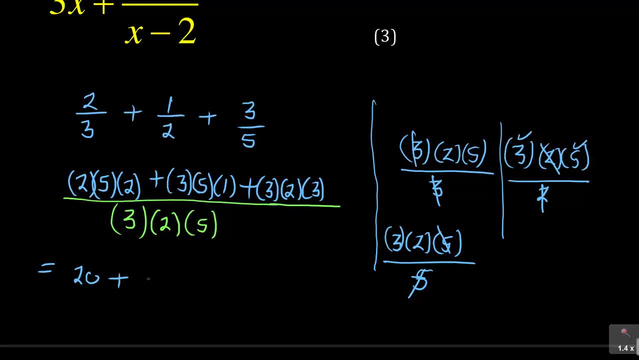 two, you have got twenty, plus three times five, times one, which is fifteen, plus two times three, which is six, six times three, which is eighteen, and then over you can even multiply now the bottom, which is three times two, which is six, and six times five, which is thirty. 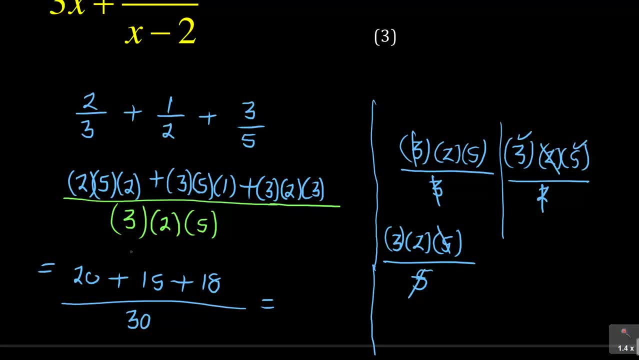 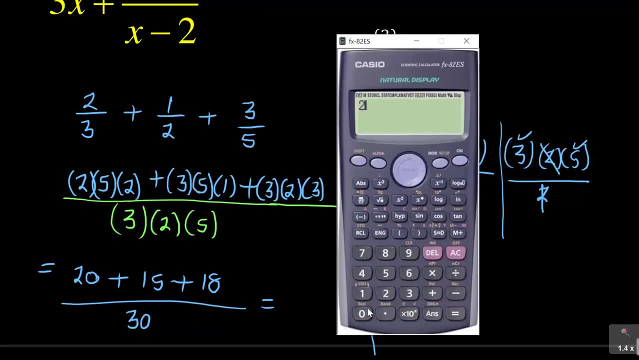 in that case. so that is what um you are having there. so now you can add in, in this case the 20 plus 15 plus 18.. i'll just quickly use the calculator: 20 plus 15 plus 18.. it gives me 50. 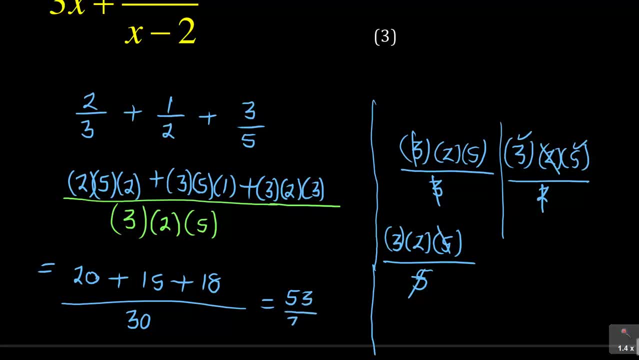 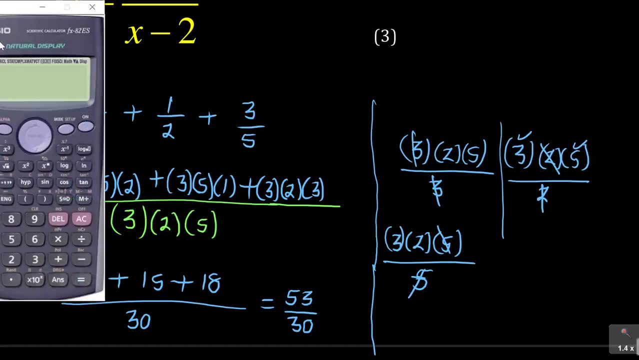 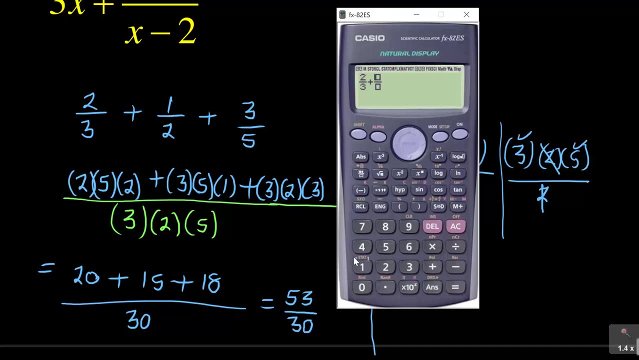 and the number that comes out is 53. so this will be 53 over 30.. i don't think there is any number that can actually simplify this feather, but i can test this with my calculator to say two over three, just to see if i'm correct, plus one over two. 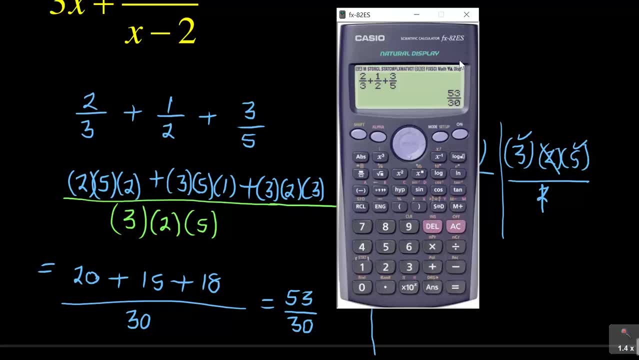 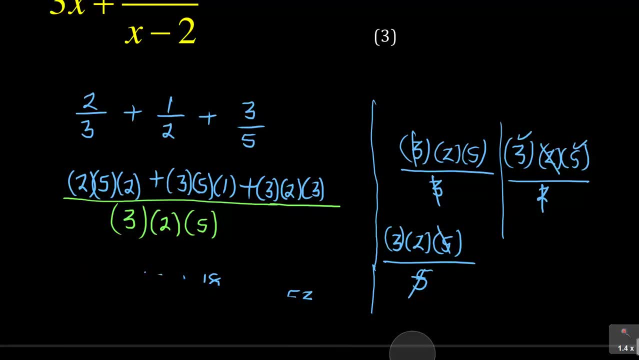 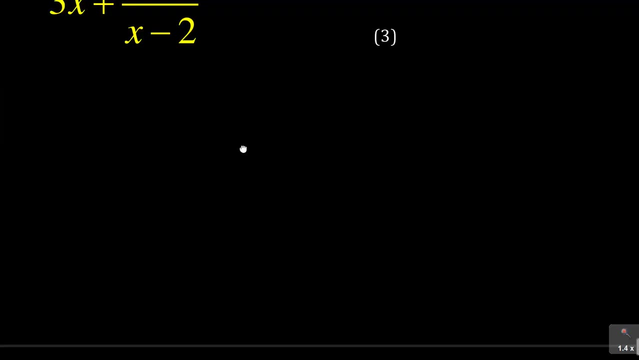 and i've got plus three over five. so if you can test this equal to, i'm getting 53 over 30.. so for this concept that i used here is the same concept that i'll use now when i'm going to be focusing on algebraic fractions. so, using the same method, let us look at this question now. i'm given a 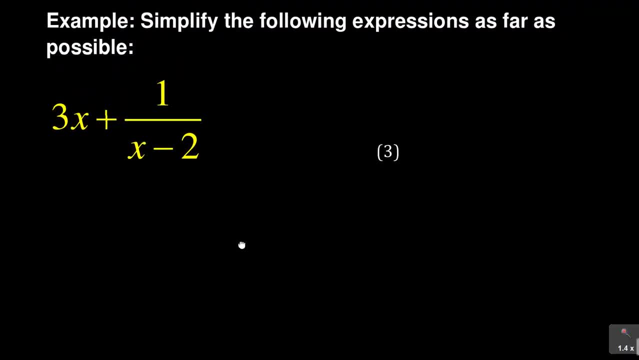 fraction says: uh. simplify the following expression as far as possible, and i'm given that. so the first thing i have to identify 3x. i must divide it by 1 so that there is fractions on each and every item. so what i have here, my common denominator, it is 1 and it is x minus 2, so i'm going to be taking that. 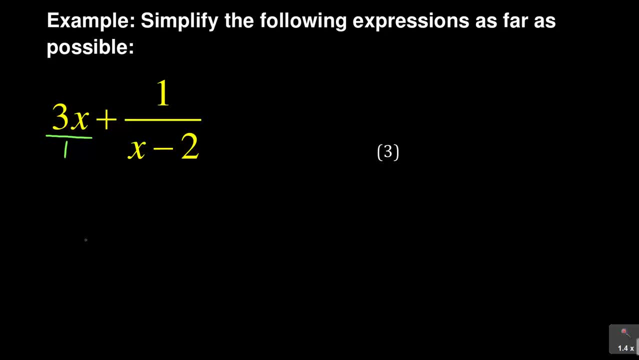 and you know 1 is simple, a 1. but just for the sake of maintaining the method that i showed you. so you take 1 and you take x minus 2. so, whatever i'm doing, i'm saying here 1 x minus 2, i'm going to divide it. 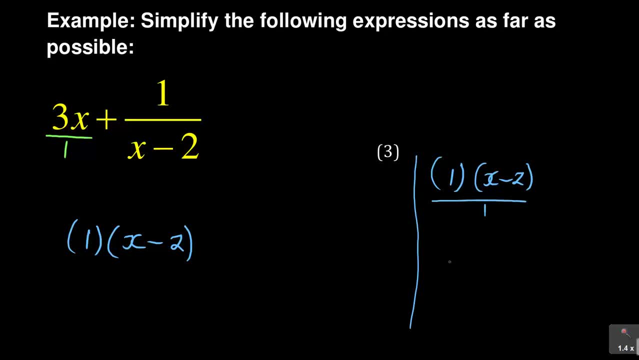 by the first one, which is 1. so this is over 1 and i've got again 1 x minus 2. i'm going to divide it now by x minus 2, so it will be that x minus 2. so when i start, uh, dividing on the first one, the 1 will cancel the 1 and x minus 2 will remain. so i will have 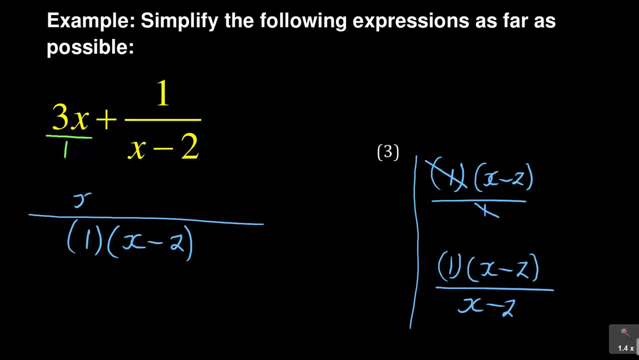 in this case, on top i will have x minus 2, remember, in bracket and then i'm going to multiply by the top and that top is 3x. so i'm going to multiply by 3x, but it is not usually more advised able to write 3x on the other side. it's better to start with 3x on this side. 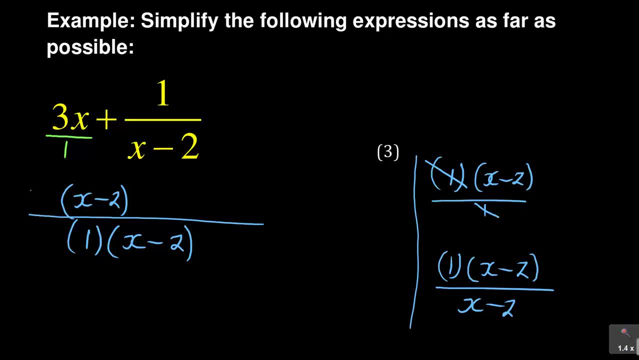 so what i'm going to have then i'm going to have my 3x here, like that it's easier to expand from that angle. then i've got a plus. i'm here now. then what i have is the x minus 2. canceling the x minus 2, the 1 is remaining, so I've got 1 in bracket. 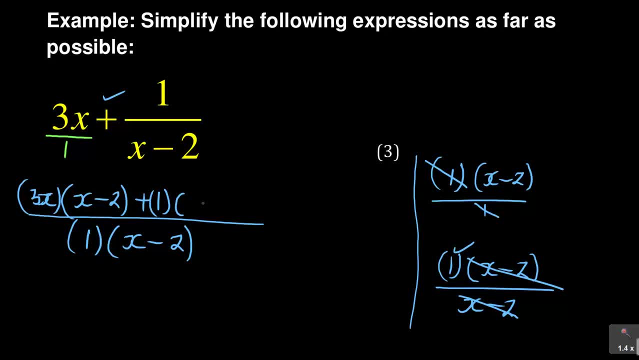 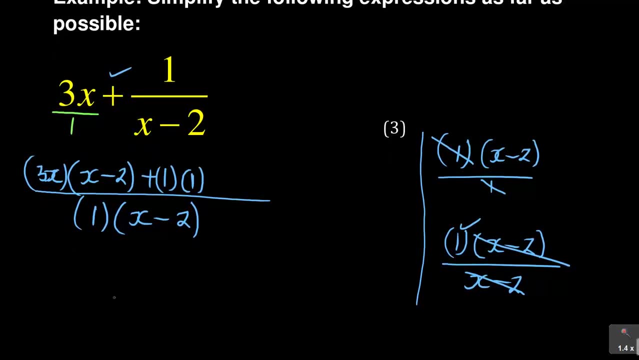 multiplied by the top there, which is a 1. so you see, I'm following, as I said, exactly the same steps that I used in the beginning. so this is equal to now. the 3x will multiply is now an expansion where the 3x will multiply the x, which is 3x times x, and the 3x will multiply. 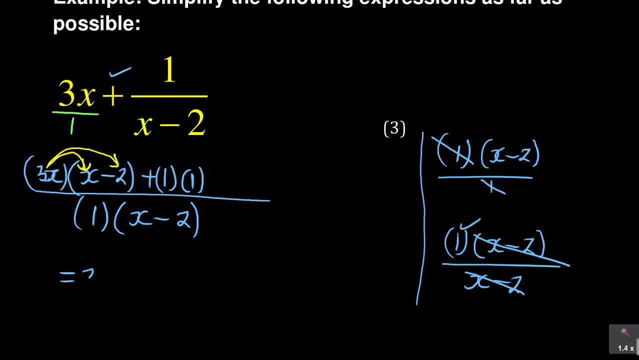 the negative 2. so 3x times x, I've got 3x squared. and then 3x times minus 2, I've got minus 6x. and then plus 1 times 1, I've got 1 over 1 times x minus 2. it will simply be x. 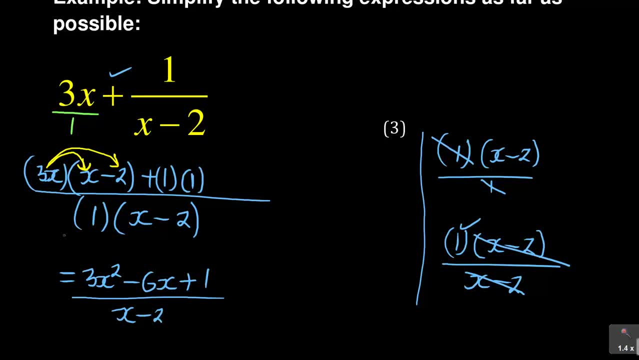 minus 2.. so this is what i am having in this case now. what is most important now is to check, if ever, is it possible to factorize the top, which is 3x squared minus 6x plus 1.. so in this stage, 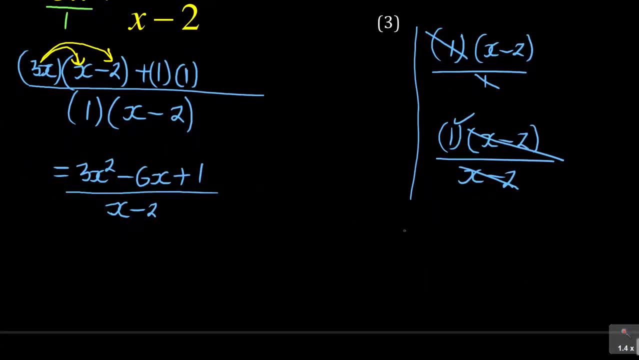 we are going to use the product sum and now i'm not going to dwell much on the product sum method, but the early sense, if you can check that, focus on product sum where i use it when i'm factorizing. so i have got 3x squared just to see if ever that can be factorized, 3x squared minus 6x plus 1, and 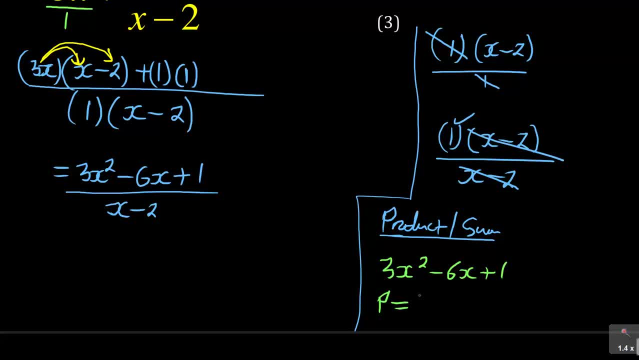 then my product. there is 3x squared times 1, which is positive 3x squared, and then my sum in this case is negative, 6x. and then i look for factors of the product, factors of 3, which is 1 times 3. 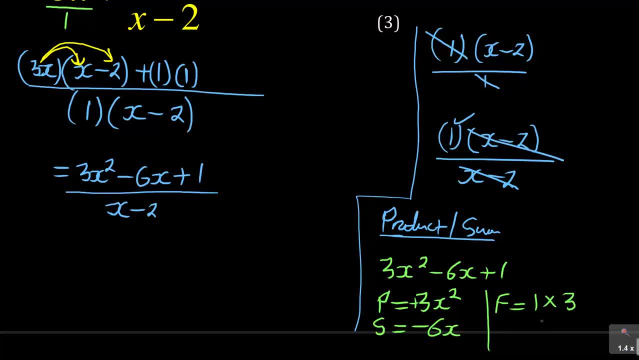 because these are the factors of 3 and there is no any other factor of 3. so i'm looking for two numbers. when i multiply them, i must get a positive 3, when i add them, i must get a negative 6.. so 1. 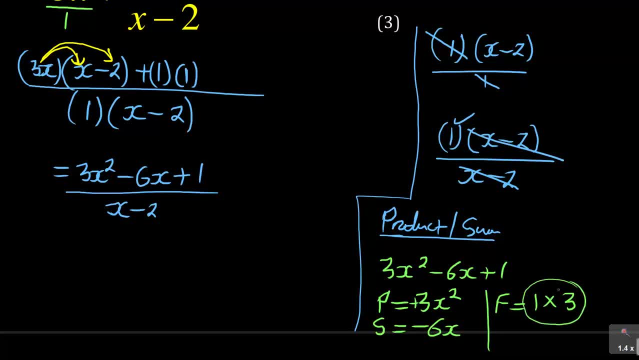 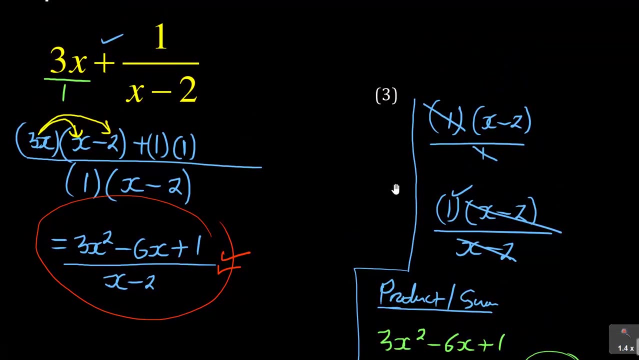 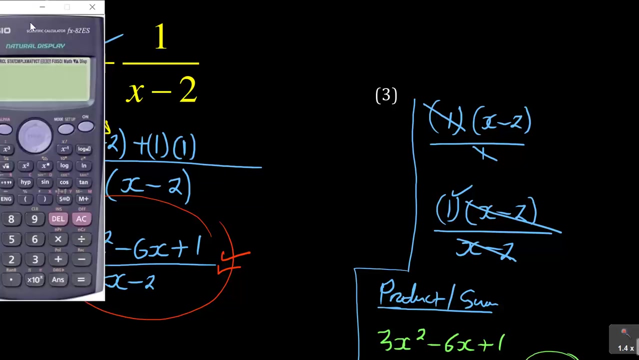 and 3 cannot give me a 6 when i add them. therefore, this becomes the final answer on that. so this is the simplified version of that. now, how do i actually test it? what i do? i go to the um in this. i take my calculator and with the calculator i got to choose any value of x, for example. let's say um. 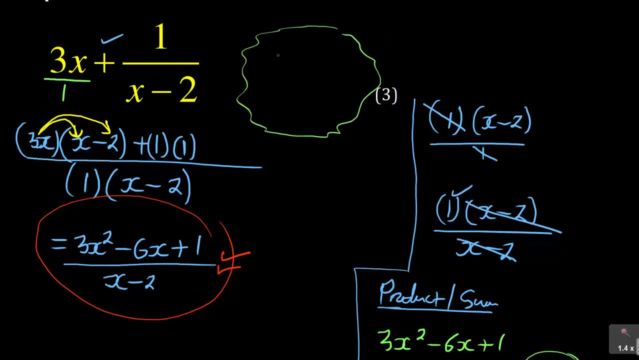 i just want to choose any value of x and say let x be equal to 4, just yeah, let's just say let x be equal to 4.. now i'm going to test with: x is equal to 4 here. and i'm going to test again with. 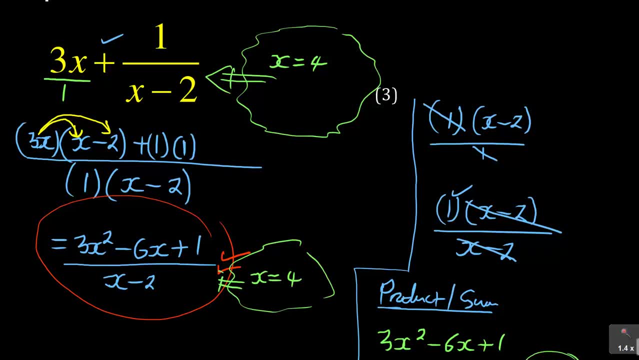 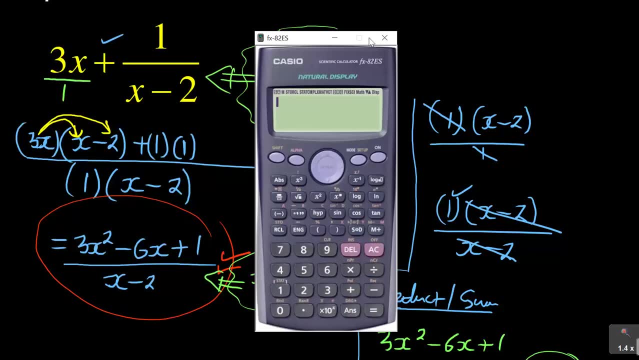 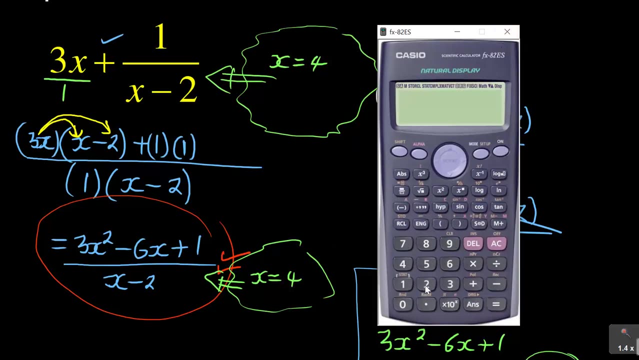 x is equal to 4 in this part. so i'm going to test with the x equal to 4 now. if the answers are matching, it means my simplification is correct. so when i do that, i'm taking this a little bit slower so that, um, when i do the second part, you'll be able to know why i do what i do. 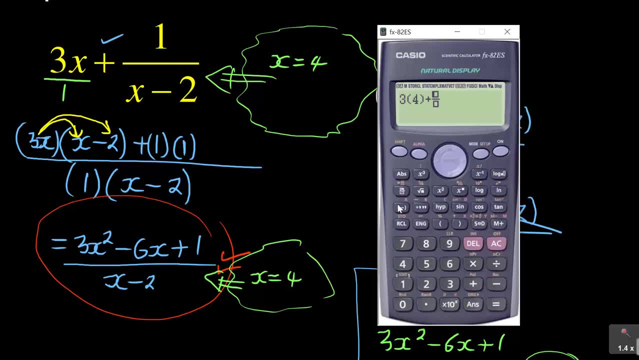 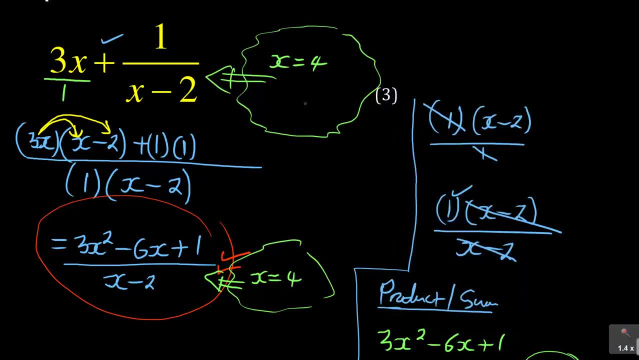 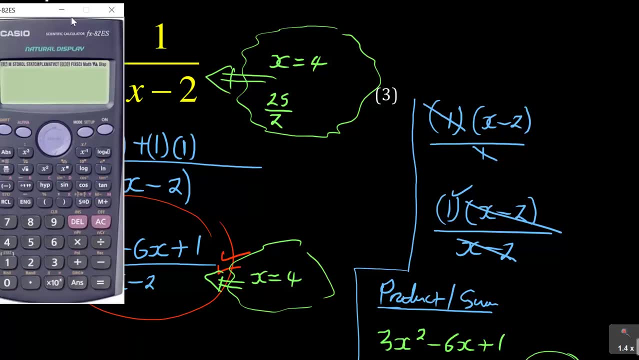 so i said x is equal to 4 plus 1 over which is 4 minus 2.. So the answer is 25 over 2.. So here I got 25 over 2.. So let's do the other one Now where there is x, remember I put a 4.. 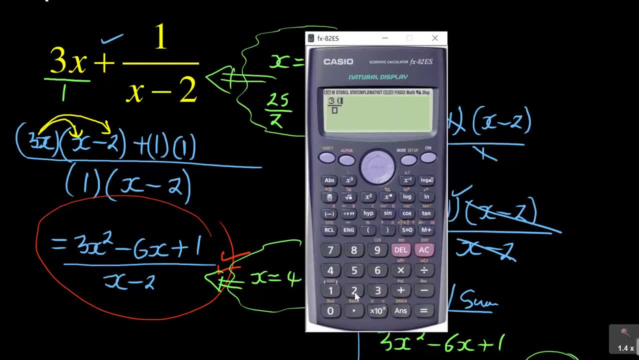 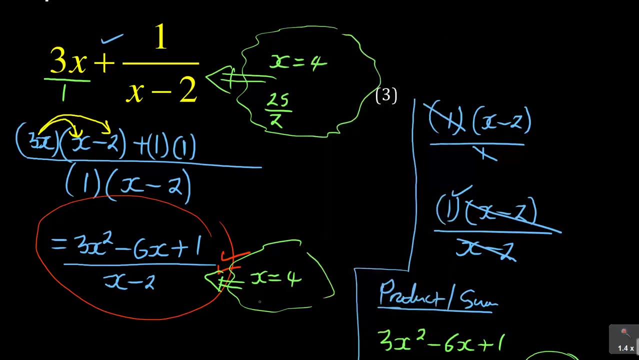 So I've got 3 into x, which is 4 squared minus 6 into 4 plus 1, all over 4 minus 2.. And then I'm getting 25 over 2.. So you can see that I'm getting 25 over 2 on both cases.